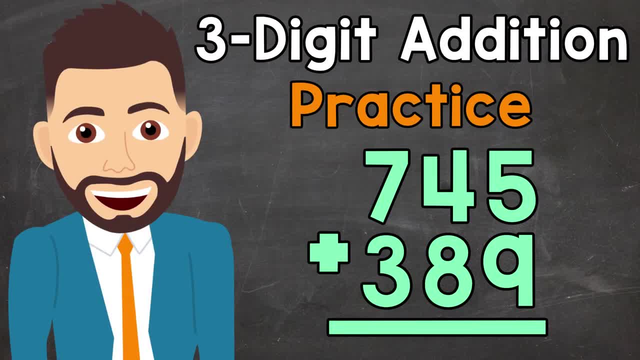 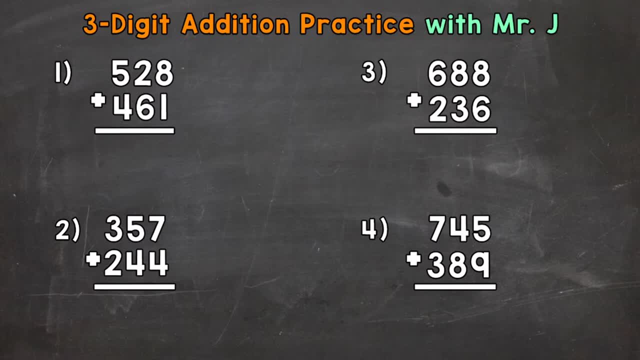 Welcome to Math with Mr J. In this video I'm going to cover some addition practice problems. Now you can work through these problems with me or feel free to press pause before I start solve the problems. when you're ready, press play and check your answers with mine. 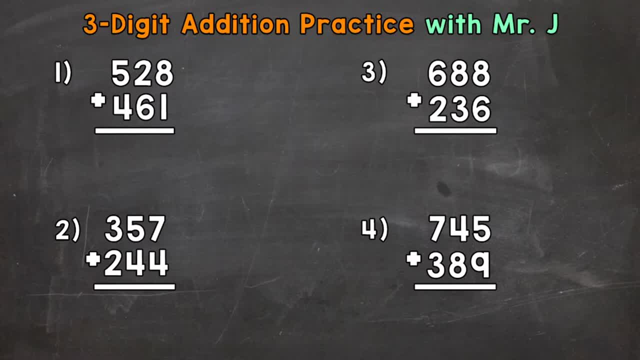 Now I do want to mention that some of these problems do involve regrouping. This is also called carrying. so to regroup or to carry, they mean the same thing. I'm going to use the word regrouping throughout this video. 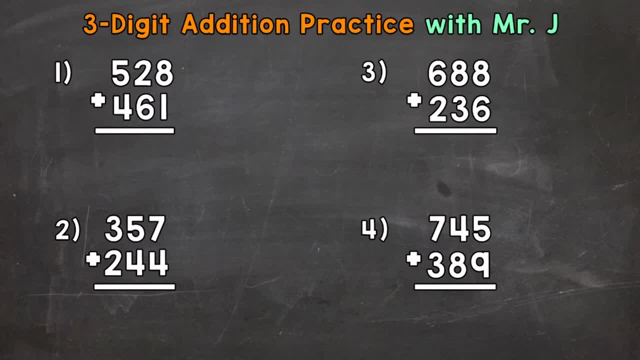 Let's get started Now. in this video, we're going to be working with three-digit numbers, So let's jump into number one, where we have 528 plus 461.. And when we add whole numbers, we always start with the ones place. 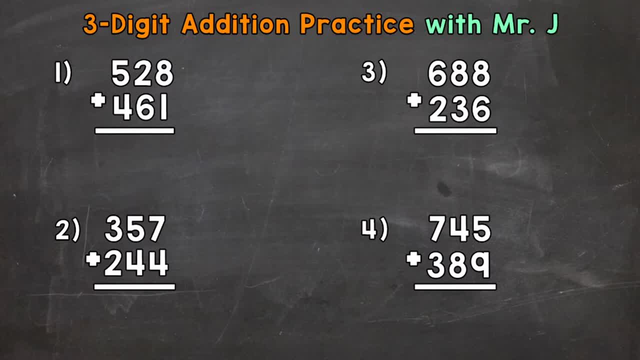 So eight ones Plus one one gives us a total of nine ones, So a nine in the ones place. Then we work our way left to the tens place. So we have two tens plus six tens, That's a total of eight tens. 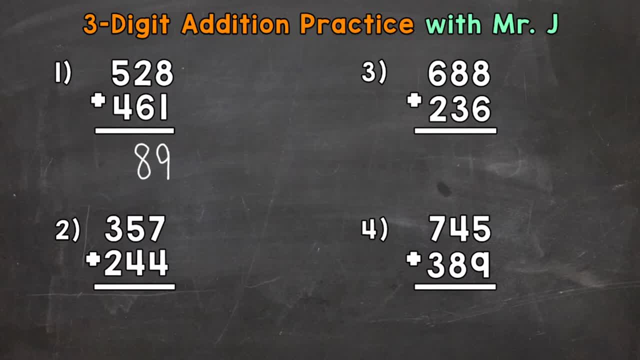 So an eight in the tens place. Now we add the hundreds place, So five hundreds plus four hundreds, Five plus four gives us a total, So a nine in the hundreds place, And our final answer is 989.. Moving on to number two, where we have 357 plus 244.. 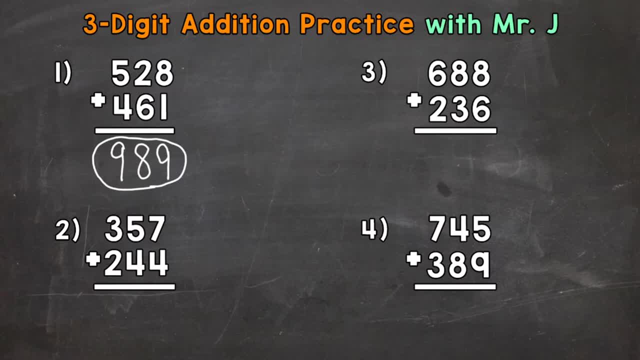 Start with the ones place. So seven plus four is 11.. We put the one from the ones place in the ones place in our answer and then regroup the one in the tens place. So we add the ones place from 11 into the tens place within our problem. 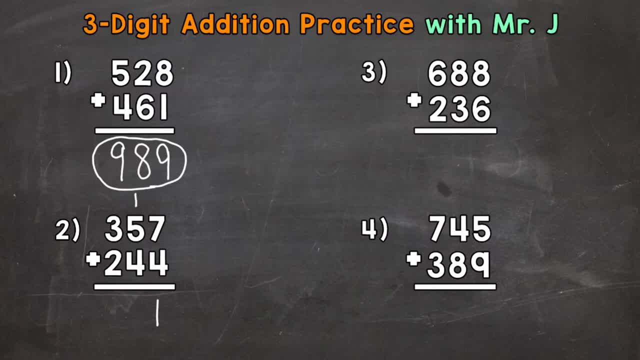 Now we add our tens, So 110 plus five, tens plus four, tens. One plus five is six plus four is ten. So we put the zero from ten in the tens place and regroup the one. Now we add the hundreds.